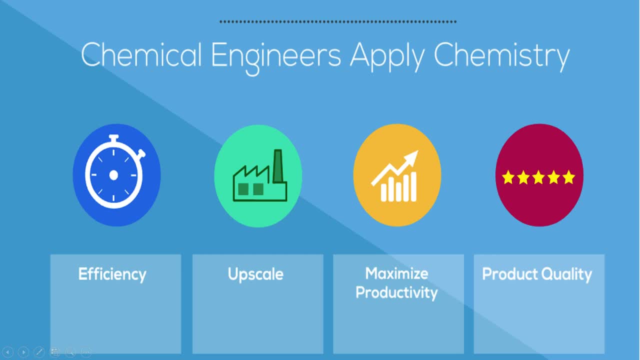 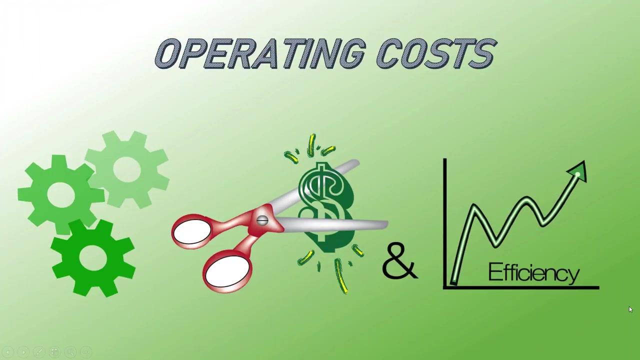 Chemical engineers take the existing chemicals and processes and really focus on upscaling the process while maintaining efficiency and maximizing productivity. Another really important role chemical engineers must take on is quality control. Chemical engineers have to focus on all these factors while also minimizing operating costs. 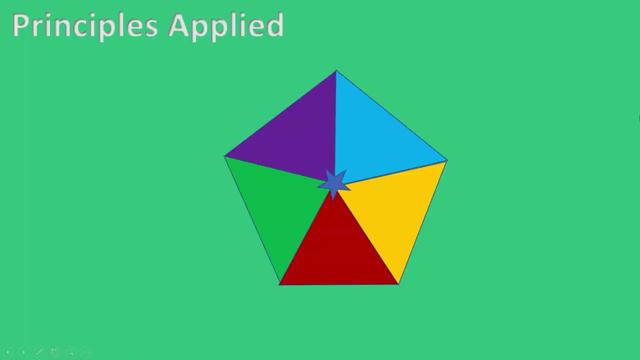 So, in order to excel in all of these roles, chemical engineers must learn and apply various principles. Chemical engineers, throughout their undergraduate and graduate-level curriculum, must fully understand the basics of chemistry, thermodynamics, math, biology and physics. In order to excel in all of these roles, chemical engineers must learn and apply various principles. 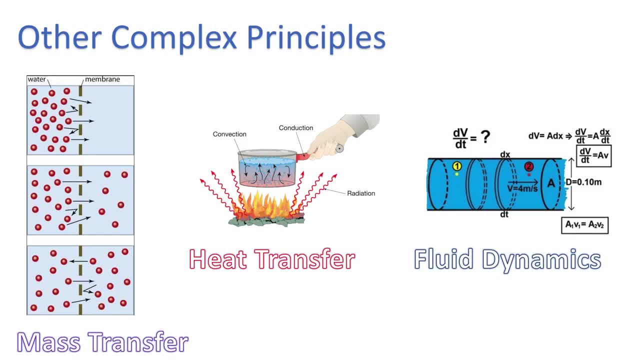 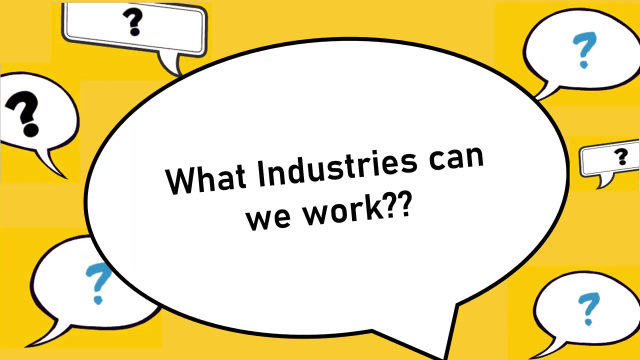 In order to excel, they also must go into other complex principles, such as mass transfer, heat transfer and fluid dynamics. All of these critical skills are needed in chemical engineering in order to really improve processes that will help most of society. So when we learn all of this, you wonder: well, what industries can engineers work in? 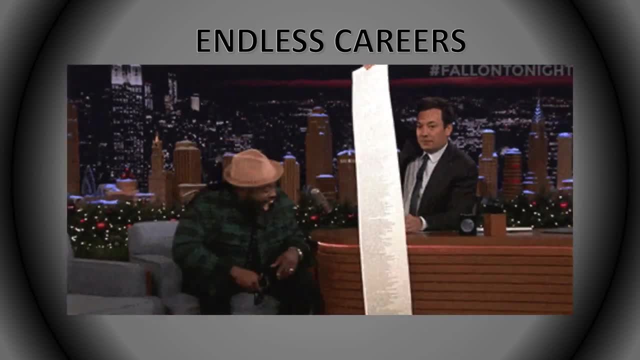 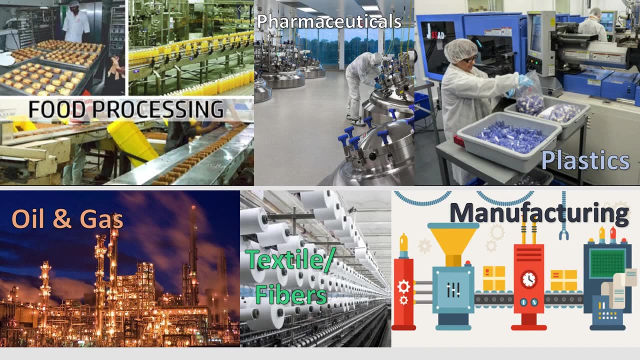 Well, the answer is: there are endless careers. We have to learn so much and understand so many fundamentals that we can go into various industries. For example, some industries involve the food processing, where chemical engineers improve the processing techniques as well as the quantity and quality of the food available. 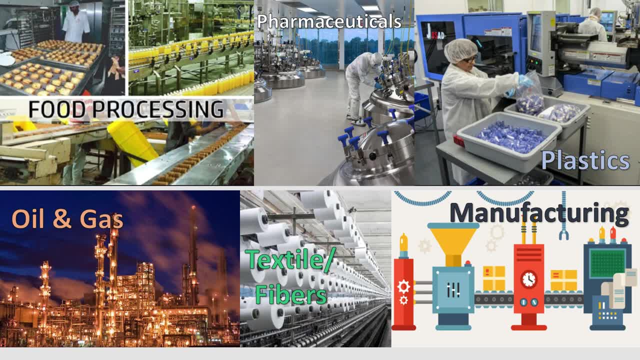 They help mass-produce drugs in the pharmaceutical industry to help them be more affordable. They can work in the plastics industry And even oil and gas Chemical engineers can go into upstream, midstream or downstream and really help make efficient methods of refining petroleum products. 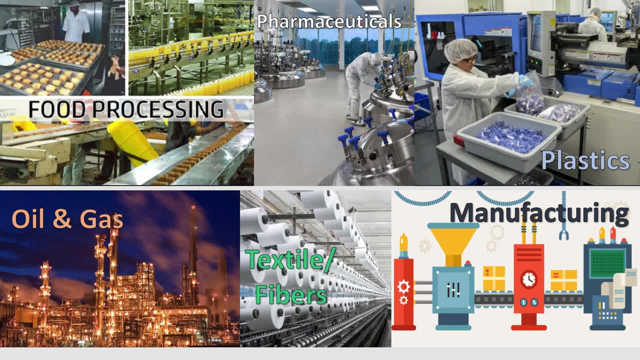 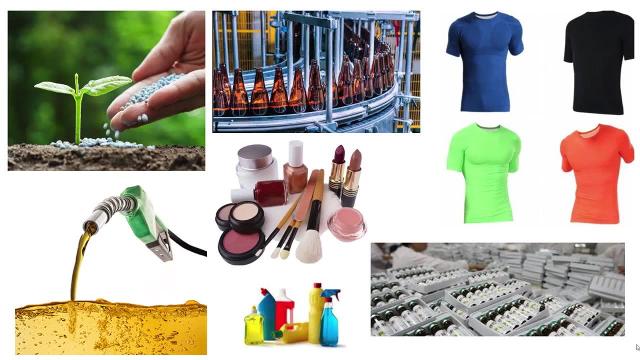 Another diverse industry chemical engineers can work in are the textile and fibers. A lot of these fibers go into the everyday clothing that we wear And, essentially, any manufacturing experience or plant a chemical engineer is able to work in. So, as you can see, chemical engineers can work in a variety of industries.